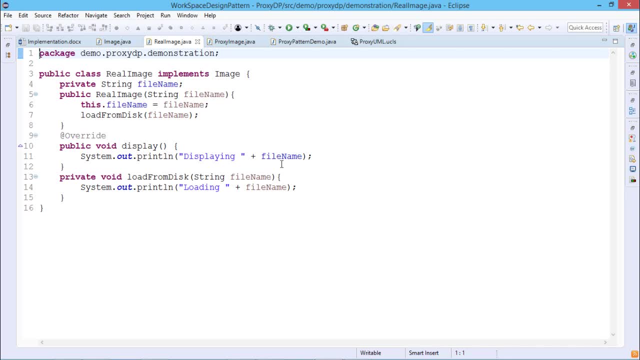 Java. so now we are going for this real image dot Java, which is implementing this image, and it is having the private string file name and public real image. so that is a constructor. here we are passing this file name as input parameter. this file name will initialize or instantiate this instance variable. 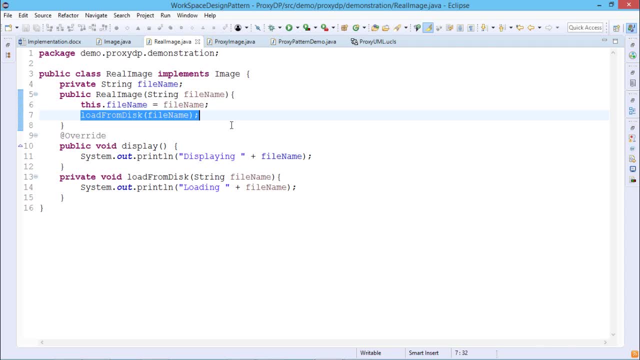 file name and load from disk will take place. so load from disk means another message will be sent to the file name and the message will be sent to the file name and the method. that is a user defined method here. member functions here, within this particular class, real image which takes this file name as input argument and. 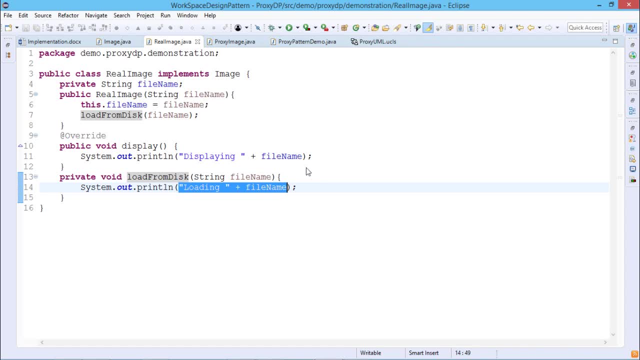 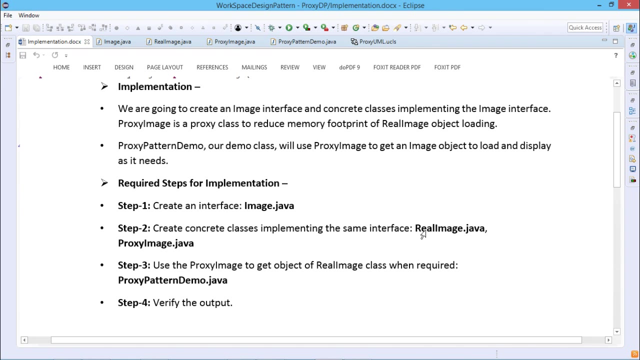 which prints this respective string. there is a loading concatenation file name. so that is my real image constructor. we are having another method that is a display and which is displaying the file name. next we are going for this proxy image. so now we know that we have discussed this real 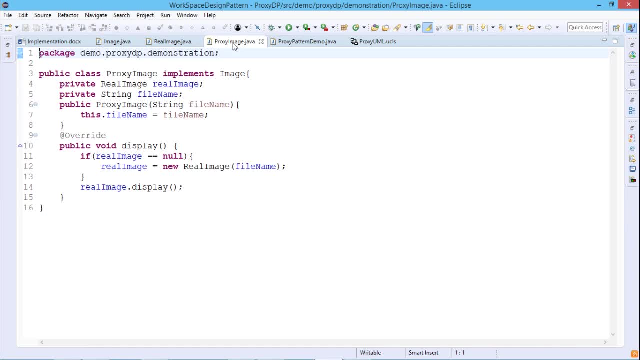 image. so let us go for this proxy image dot Java and proxy image dot Java. so let us go for this proxy image dot Java. in case a proxy image dot Java, it is also implementing this image interface. so as a result of that, this display method must be defined here, overwritten here. so 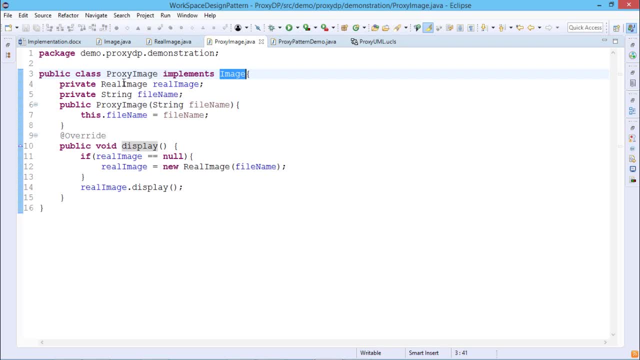 it is also having one instance variable of the type real image. there is a real image, so string file name. so proxy image is a constructor, so string file name will be the input parameter. this dot file name- that is a instance variable file name will be in- will be initialized with this input parameter file name. so 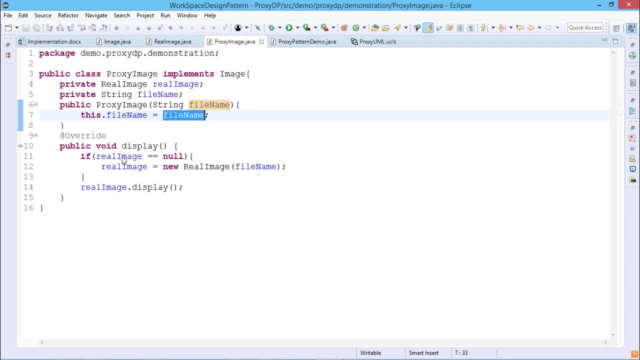 here we are having this display and display is telling that if real image is equal to is equal to null. that means if the real image is null, then a new real image will be created against the file name. otherwise the real image dot display will take place in both cases: if the real image is equal is equal to null, or if 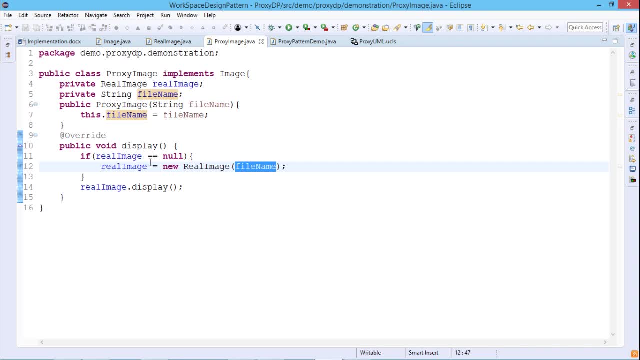 the real image is not equal to null. in both cases the real image dot display will be printed. that means this very method will be executed. so there is a systemoutprintlnDisplay concatenation, the file name. so let us go for this proxy pattern demo. so in the 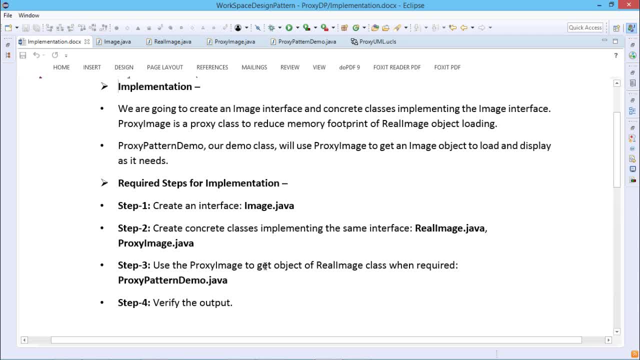 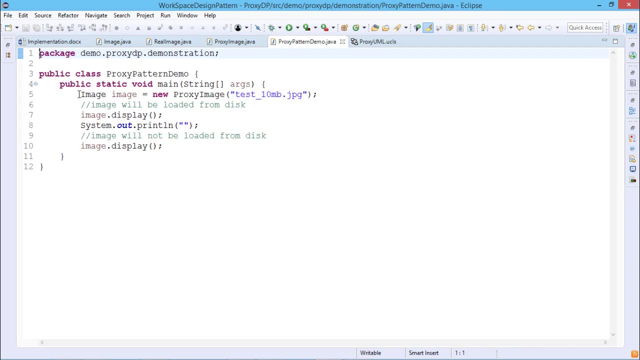 implementation. we are having the step number three: use a proxy image to get object of real image class when required and that will be shown in case of proxy pattern, demo dot Java, and verify the output. so there is a proxy pattern, demo dot Java. here we are having one image object, that is, the image is equal a new. 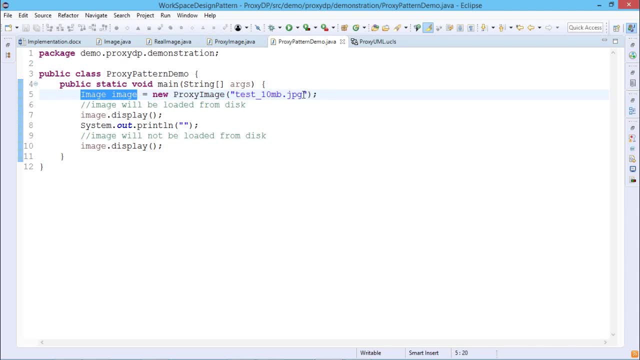 proxy image: test: underscore: 10 MB dot jpg. so there is a. there is a one image object, image class object, image interface object. we're going to create and it is getting instantiated using this new proxy image. there is a constructor passing this file name here as input argument, and then you shall go. 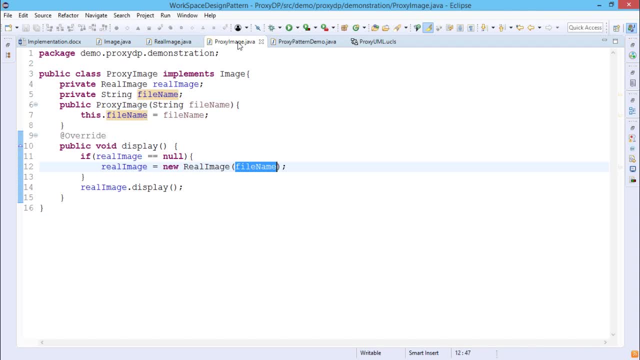 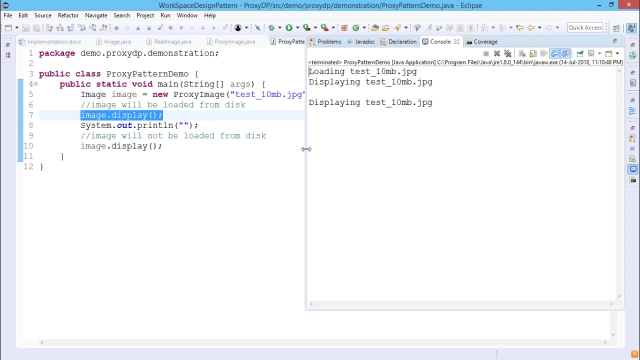 for this image dot display. we know that in case of proxy image, for the first time, this real image object- there is a real image- will be equal to null. so as a result of that, this real image will be instantiated here. so now what will happen? now let me go for the output. so here you can find that, this output. 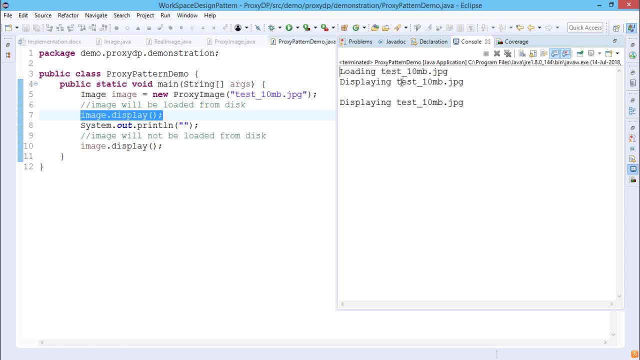 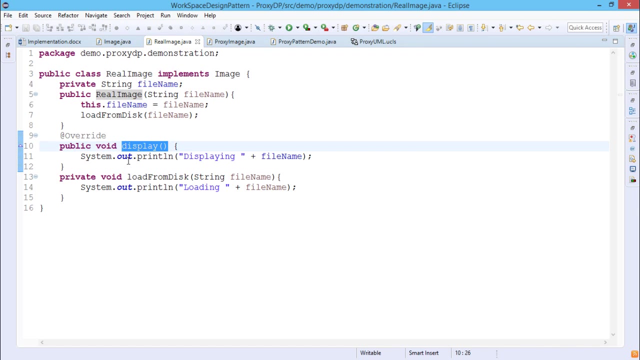 loading test at 10 MB dot jpg and displaying test underscore: 10 MB dot jpg. so loading means so. loading means you can find that here, in this case, if this real image is equal to, is equal to null, it will go for this constructor and in this constructor, in this constructor, load from disk this. 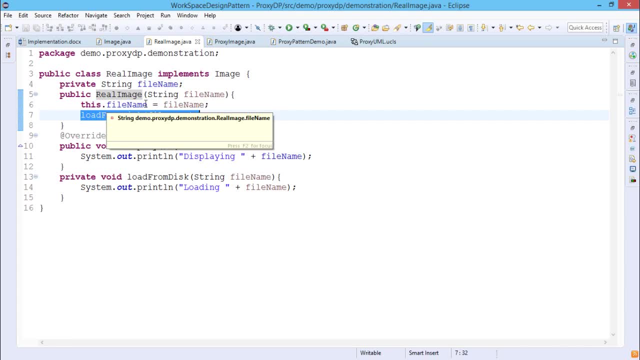 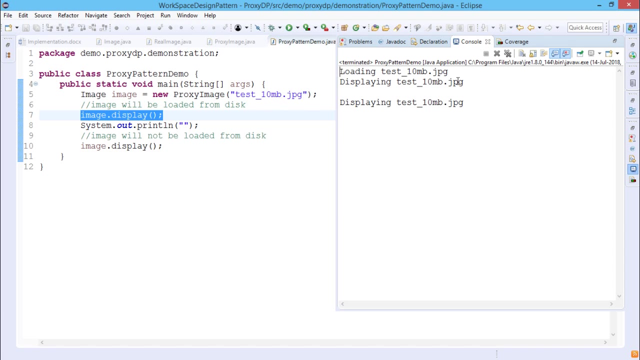 particular method will be called after instantiating this file name. there is a member variable and in case of load from image, this loading plus file name will be printed, so you are getting the same output here. you can find that. so loading plus file name is getting printed and then displaying the file name is getting. 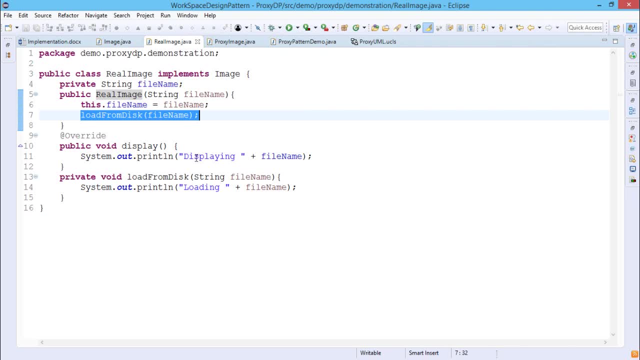 printed. so displaying file name is there. so there is a display file name. you know that whenever we are going for this, this particular proxy image, the display method is being called. so real image dot display is getting. real image dot display is getting called here. so, as a result of 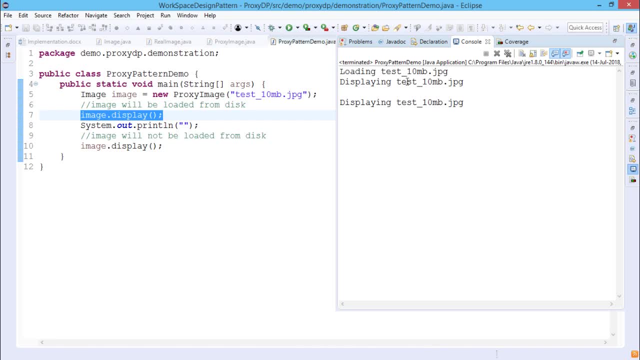 that we are getting this particular message. that is my displaying file name. but when we are going to create, when you are going to call this display method for the second time, as this real image is is now having the instantiation. so loading file name, that is a loading from disk, load from this, that method will 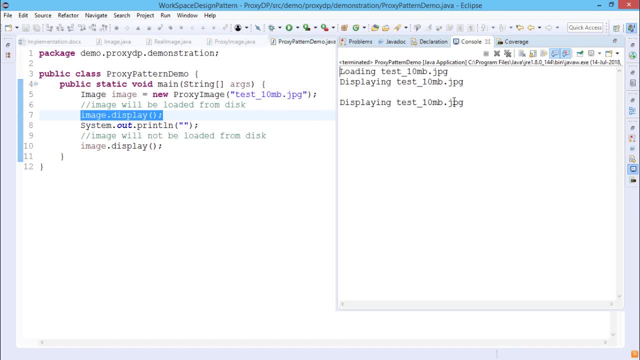 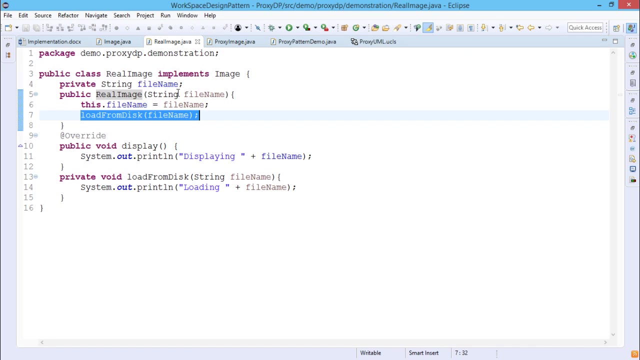 not be executed, so displaying file name will be executed here. so that is the main theme behind this proxy design pattern, so let us go for a quick revision. so imagejava is containing this interface. you are getting this code having only one unimplemented method. display real image is actually implementing this image. 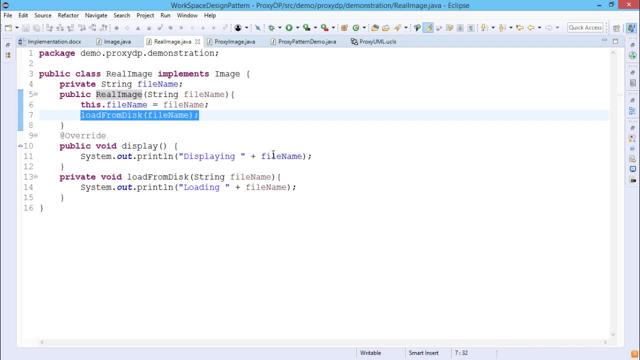 so here we are having this display method. we are going for this file name, going for this display. real image is nothing but the constructor here, so it is just instantiating this file name and load from disk is getting invoked. this method has been called load from disk is there, it is passing. 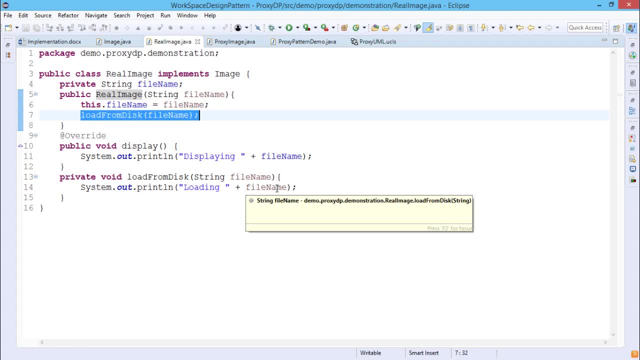 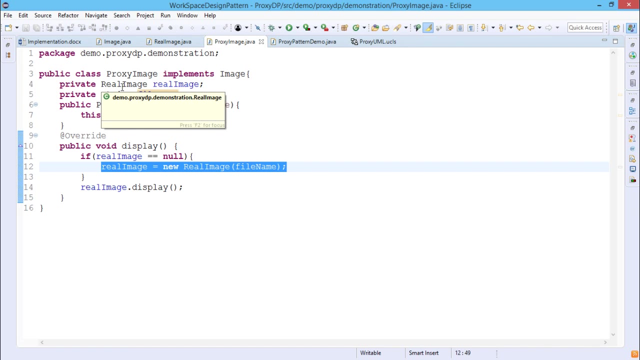 this file name as the input argument and loading concatenation file name will be the output string to be printed. and here we are having one display method displaying the file name in case of proxy image, which is implementing this image again, but taking this real image class object as instance. 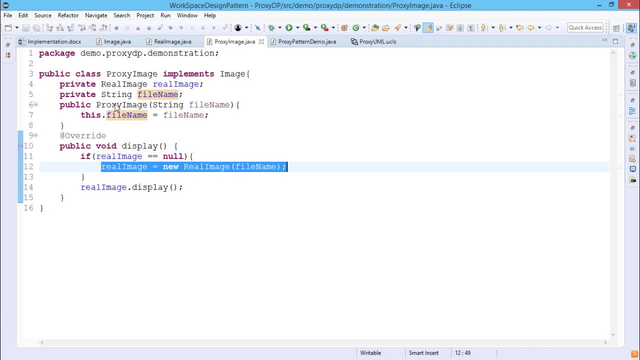 variable you can find. here we are having this string: file name: proxy image. is the constructor taking this file name as input parameter? this dot file name is equal to file name, so this file name is getting instantiated. display method has been called if the real image is already is equal to equal to null. 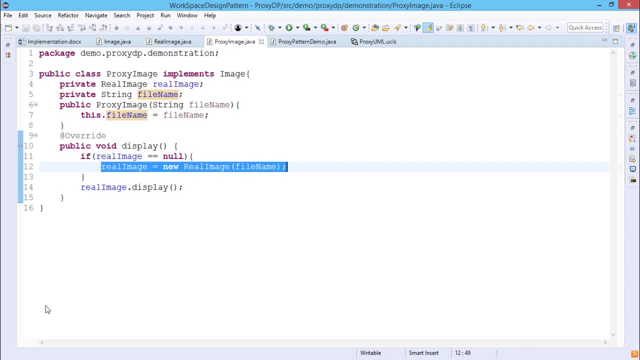 that means the real image is uninstantiated, then the real image will get instantiated. so, as a result of that, from this real image, this load, from this method will be called, and otherwise it is just this real image dot display will be will be executed. so if the real image is pre-existing, 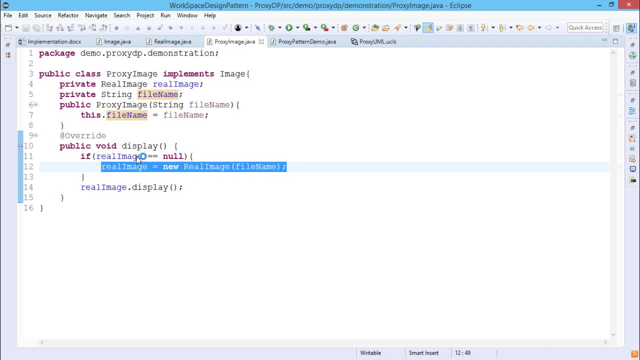 only real image dot display will be executed. if the real image is not pre-existing, not instantiated, then it will be created. then real image dot display method will be called. so here we are having this proxy pattern, demo dot java, and in this case you can find that for the first time. 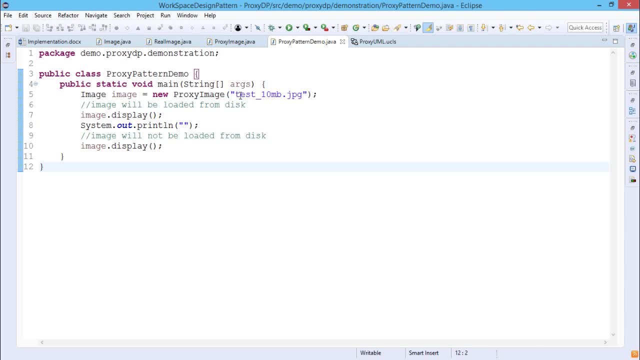 when we are calling this new proxy image with this particular file name, then this image is getting instantiated and image dot display you can find here. i'm just executing the code, so loading the file name is getting executed. and then displaying file name is getting executed when you are going for this image dot display for the second time, so displaying file name is getting. 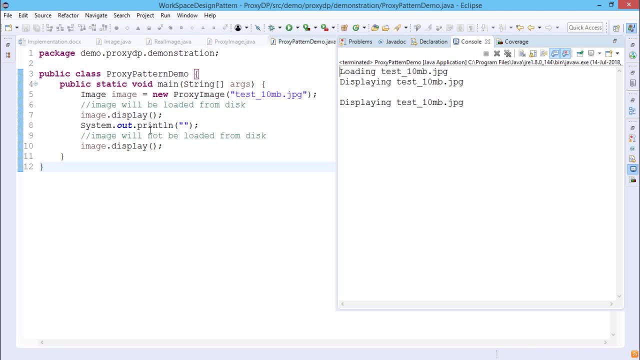 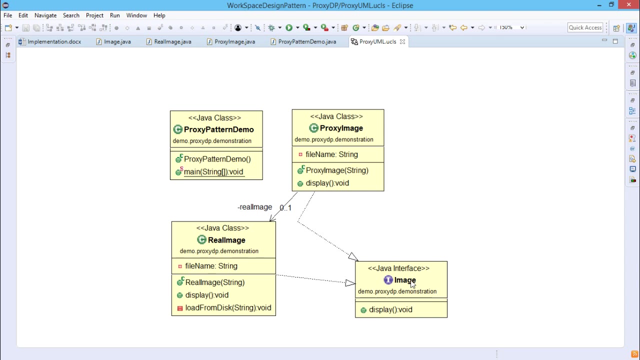 executed. so image will be loaded from the disk. but image will not be loaded from the disk because already real image object is instantiated. so let us go for the uml diagram. so there is a class diagram you are having here. so this the interface is, the is image. this interface has got implemented.